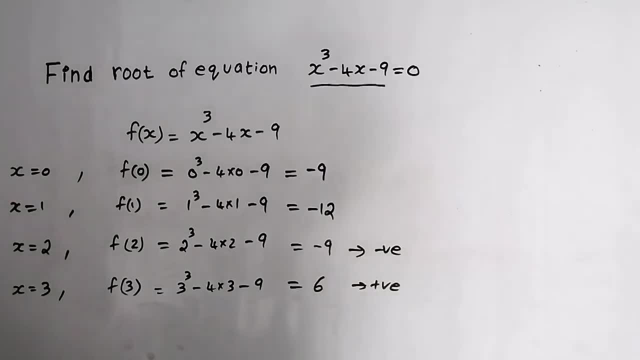 here it is a positive value. we need to get adjacent negative and positive value. so our interval, so our interval will lie between negative value and positive value. so our interval will be when x equal to 2 and when x equal to 3, and in x equal to 2 we will get negative value. in x equal to 3, we will get positive. 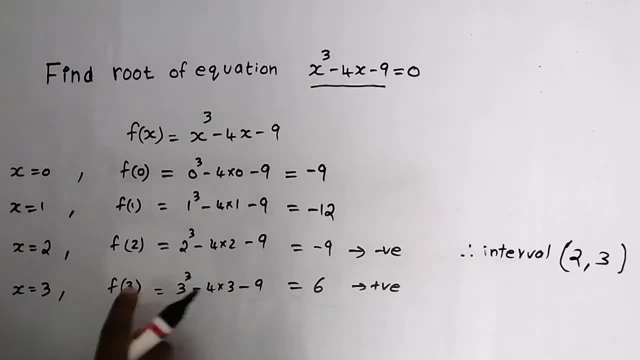 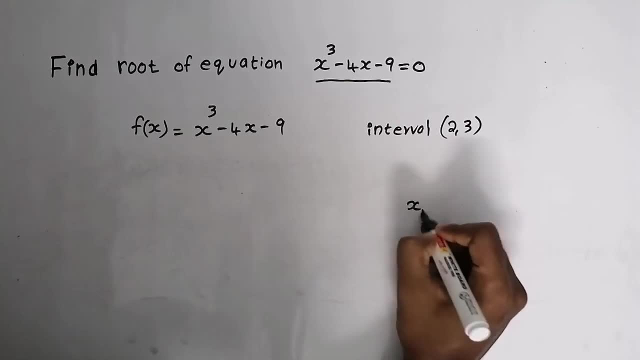 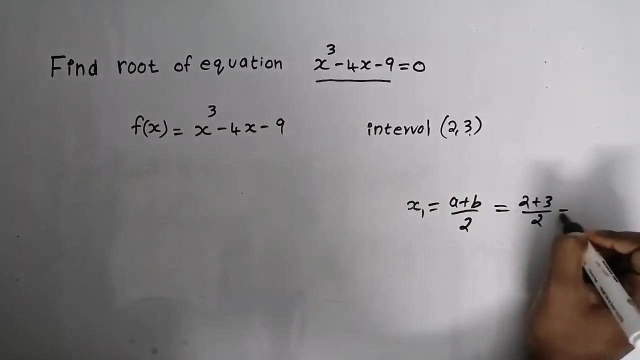 value. we need to get adjacent negative and positive value. that will be our interval. so we get the interval. that is step 1. now find the x1. that is our next step. x1 equal to a plus b by 2. so our a value is 2 and b value is 3. so 2 plus 3 by 2, that will give 5 by 2. that 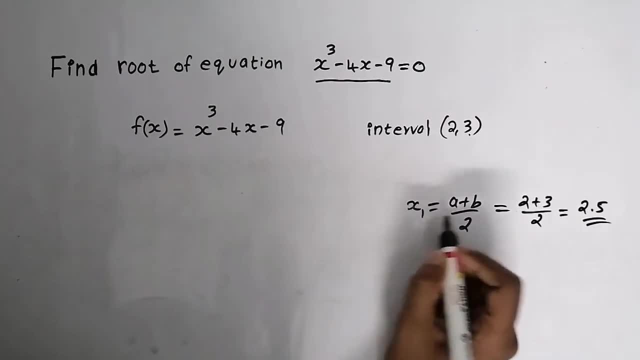 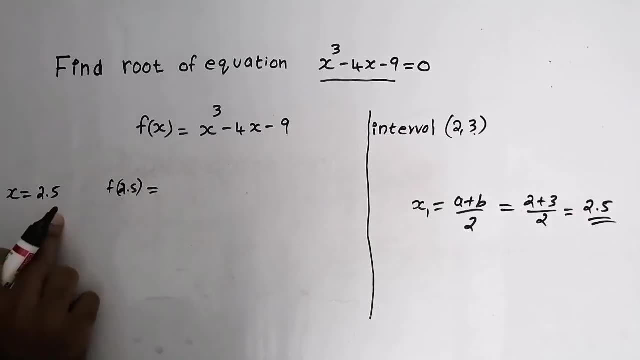 is 2.5. that is our new x1. now we got x1 equal to 2.5. so when x equal to 2.5, we need to put X in this equation. so f of 2.5, that will be equal to minus 3 point. 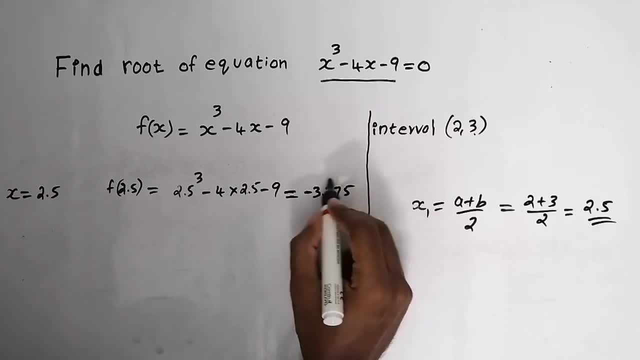 2.5. so f of 2.5 that will be equal to minus 3 point 2.5. so f of 2.5 that will be equal to minus 3 point 2.5. so f of 2.5 that will be equal to minus 3 point 375. so here it is a. 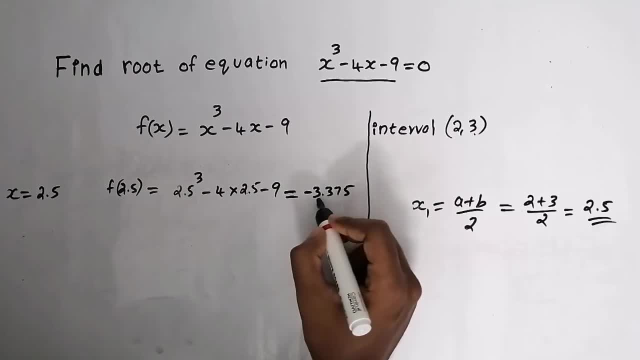 375. so here it is a 375. so here it is a negative value. if it is a negative value, negative value. if it is a negative value, negative value. if it is a negative value. replace interval a if it is a positive. replace interval a if it is a positive. 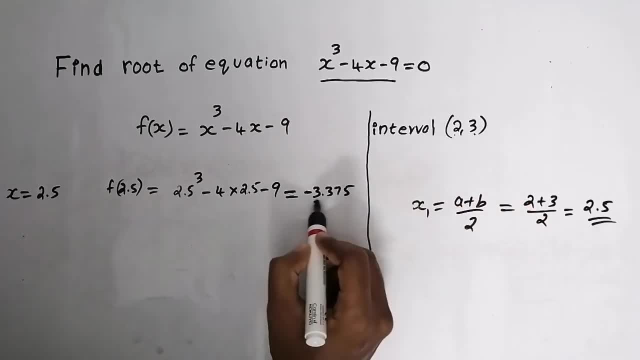 replace interval a. if it is a positive value, replace interval B. so here it is a value. replace interval B. so here it is a value. replace interval B. so here it is a negative value. so we are going to negative value. so we are going to negative value, so we are going to replace interval a, we are going to replace. 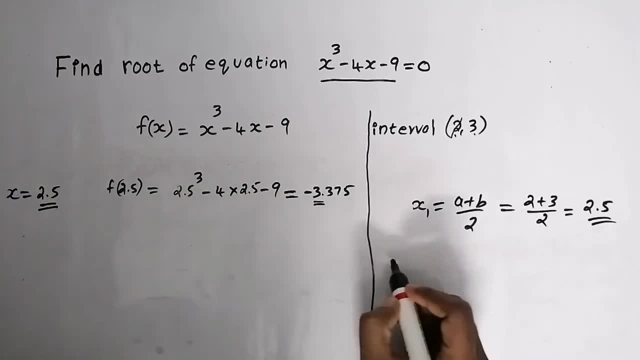 replace interval a. we are going to replace. replace interval a. we are going to replace interval a with X equal to 2.5. so interval a with X equal to 2.5. so interval a with X equal to 2.5. so our new interval will be, so our new. 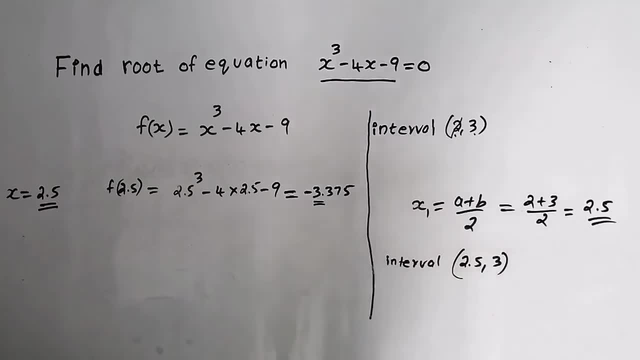 our new interval will be so our new, our new interval will be so. our new interval will be 2.5 comma 3, now do. the interval will be 2.5 comma 3, now do. the interval will be 2.5 comma 3, now do the second iteration, so X, 2 equal to a plus. second iteration, so X 2 equal to a plus second iteration, so X 2 equal to a plus B by 2, that will be 2.5 plus 3 by 2. B by 2, that will be 2.5 plus 3 by 2. 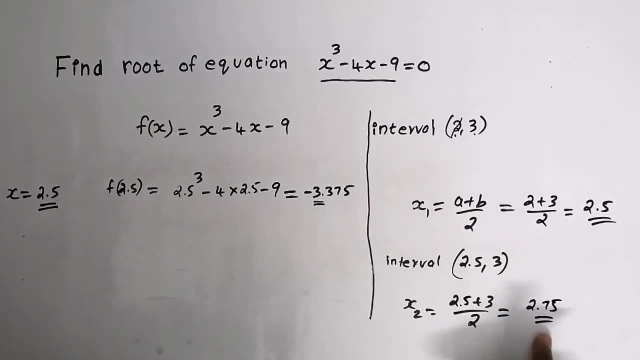 B by 2, that will be 2.5 plus 3 by 2, that will be equal to 2.75. now put X equal, that will be equal to 2.75. now put X equal, that will be equal to 2.75. now put X equal to 2.75. so now X equal to 2.75 now. to 2.75, so now X equal to 2.75. now to 2.75, so now X equal to 2.75. now do f of 2.75 substitute in this equation. do f of 2.75 substitute in this equation. 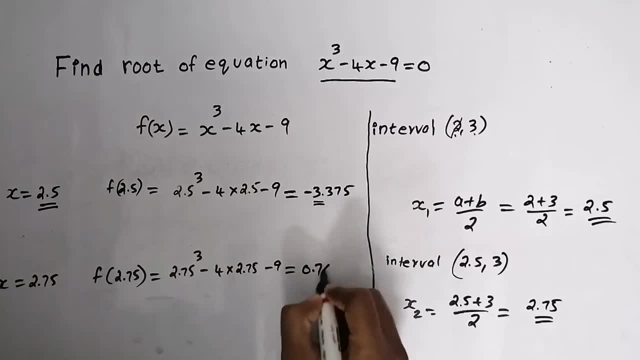 do f of 2.75. substitute in this equation with X equal to 2.75. that is equal to with X equal to 2.75. that is equal to with X equal to 2.75, that is equal to 0.76, 0.79, 6, 8. so here it is a positive. 0.76, 0.79, 6, 8. so here it is a positive 0.76, 0.79, 6, 8. so here it is a positive value. if it is a positive value, we need value. if it is a positive value, we need. 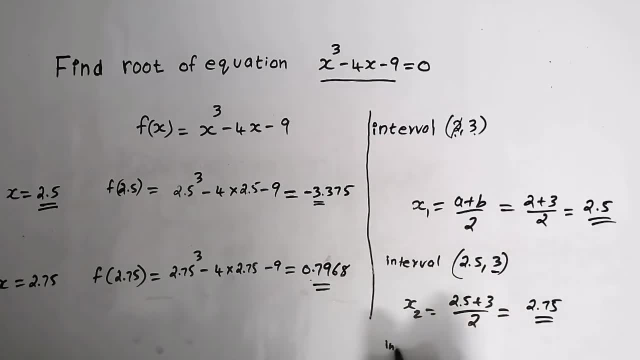 value. if it is a positive value, we need to replace interval B. so our new to replace interval B, so our new to replace interval B, so our new interval will be equal to 2.5 comma. then interval will be equal to 2.5 comma. then 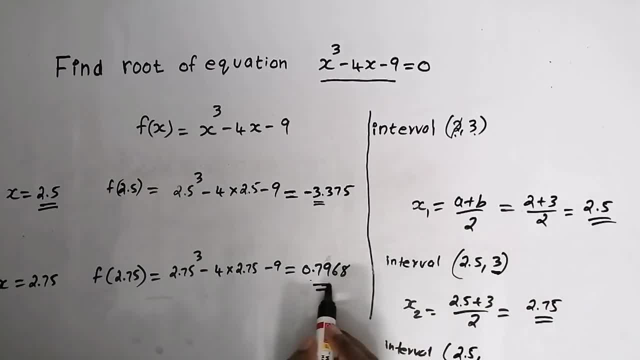 interval will be equal to 2.5 comma. then we are going to replace interval B, we are going to replace interval B. we are going to replace interval B, interval B, because our answer is a interval B, because our answer is a interval B, because our answer is a positive value. so we are going to. 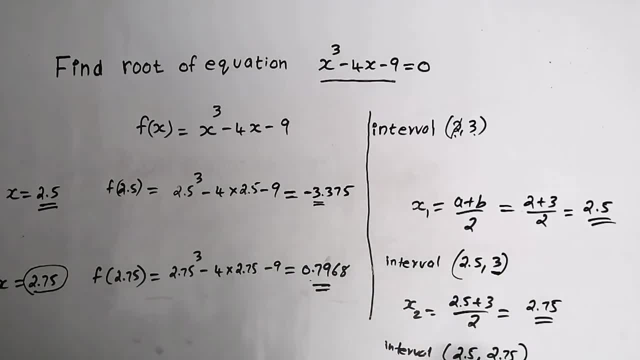 positive value. so we are going to positive value. so we are going to replace interval B with 2.75. so our replace interval B with 2.75. so our replace interval B with 2.75. so our root lies between 2.5 and 2.75, like that. 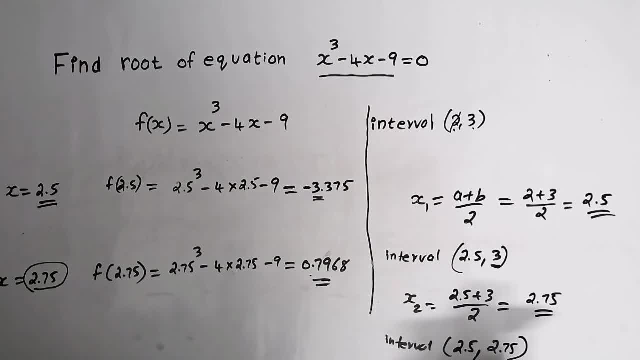 root lies between 2.5 and 2.75. like that, root lies between 2.5 and 2.75. like that, do the remaining iteration and you will do the remaining iteration and you will do the remaining iteration and you will get root between 2.5 and 2.75. so our 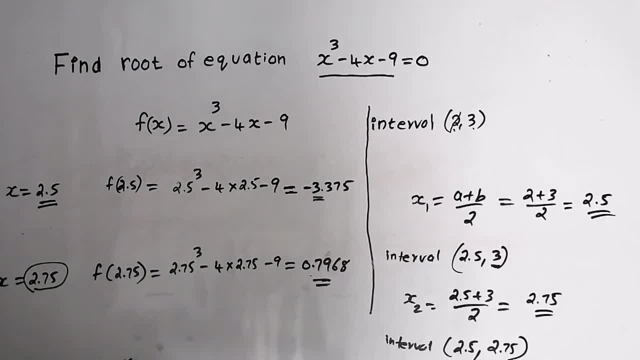 get root between 2.5 and 2.75, so our get root between 2.5 and 2.75. so our final answer will be: or root will be. so final answer will be: or root will be. so final answer will be: or root will be. so do the number of iteration as mentioned. 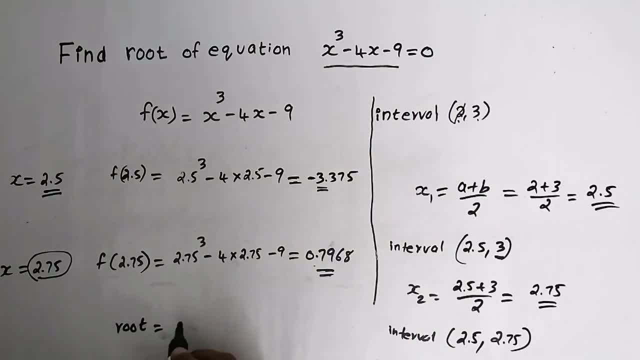 do the number of iteration as mentioned? do the number of iteration as mentioned in the question and for this question in the question and for this question in the question and for this question, the final root will be equal to 2.7, 0, 6, 5. 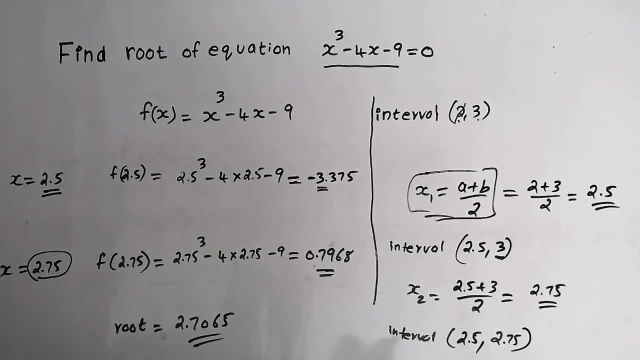 the final root will be equal to 2.7 0, 6, 5. the final root will be equal to 2.7 0, 6, 5. so do the number of iteration mentioned. so do the number of iteration mentioned. so do the number of iteration mentioned in the question. and we will get old. the. 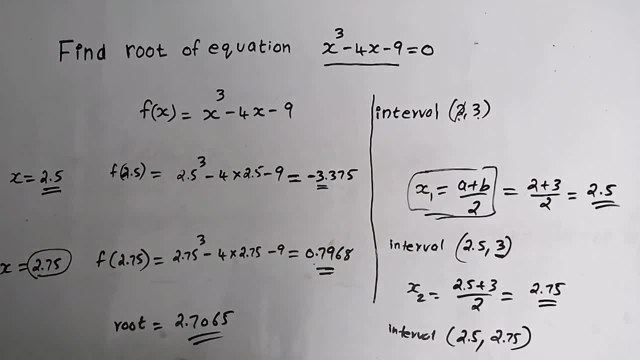 in the question and we will get old. the in the question and we will get old. the answer will be lying between 2 and 3. answer will be lying between 2 and 3. answer will be lying between 2 and 3. and here it is 2.7 0, 6, 5. that is bisection. and here it is 2.7 0 6, 5, that is bisection. and here it is 2.7 0 6, 5, that is bisection method. Welcome back to the Michigan Geological Survey YouTube channel. The following video will discuss a variety of jobs in the geosciences, including educational needs, salaries, and the typical duties of that job. The average pay and job growth were researched using the U.S. Bureau of Labor Statistics. We have grouped jobs into five categories, environmental, natural resources, academic research, engineering, and remote sensing. This list is by no means comprehensive. But we have included them in the description below, and we hope it will be a solid beginning towards answering the age-old question, what do geoscientists do? 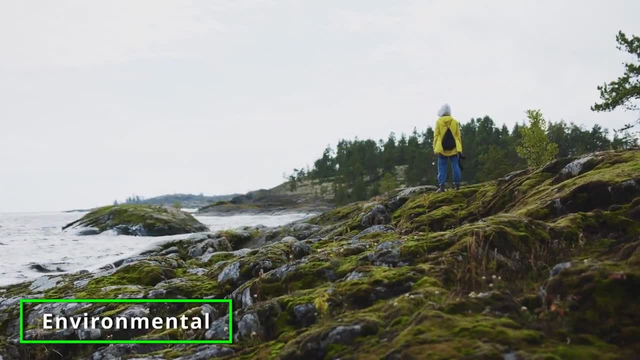 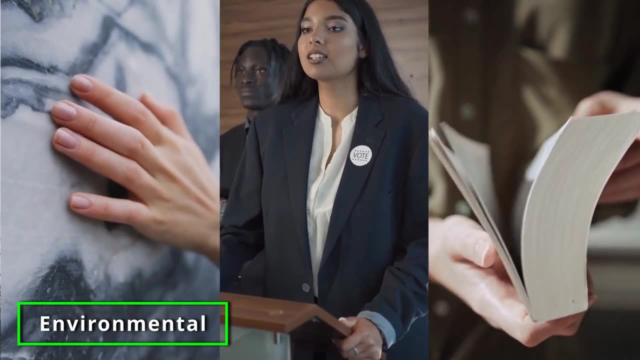 Careers in environmental sciences can vary greatly, from fieldwork careers to working in the field. We have a wide variety of jobs, including environmental science, working in policy, all the way to education. Careers often involve identifying issues in environmental regulation, energy use, ecosystem health, and recommending solutions in these areas. 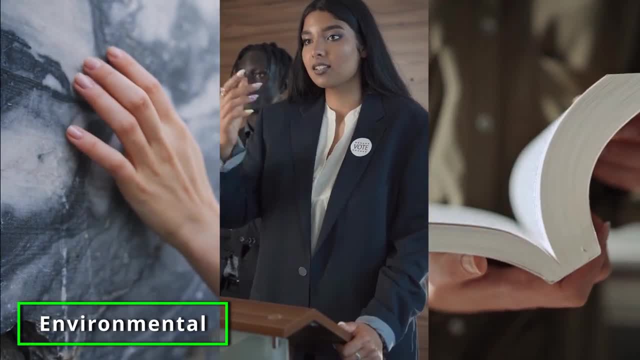 Additional subjects such as climatology, biology, aqueous chemistry, policy, and remediation can all be included when working in an environmental career. 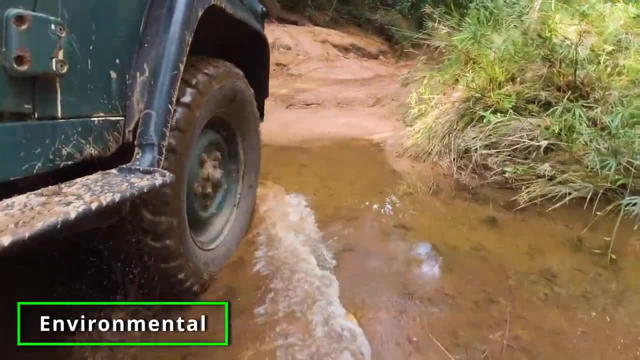 For students who like to get out in the field and don't mind a bit of physical work, an environmental field technician is a great starting point. At this job, you can expect to collect air, water, and water. This is a great starting point for you. 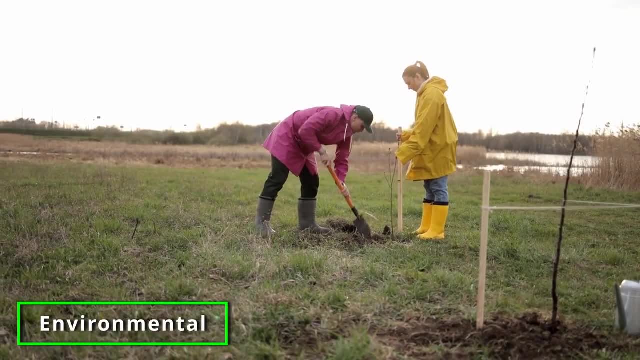 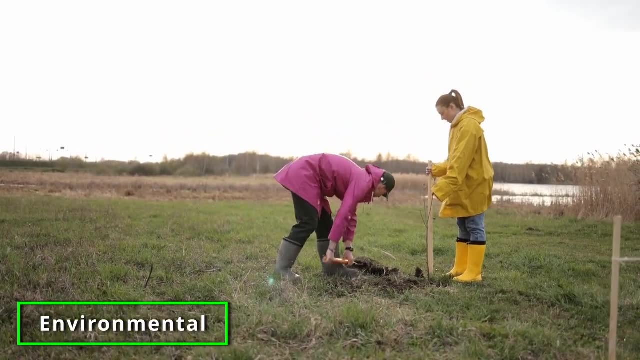 You can also get water and soil samples for pollutant assessment, prepare and clean equipment for data collection, and discuss results and write reports for clients or project managers. Many are also responsible for site upkeep, including making sure the job site is clean and 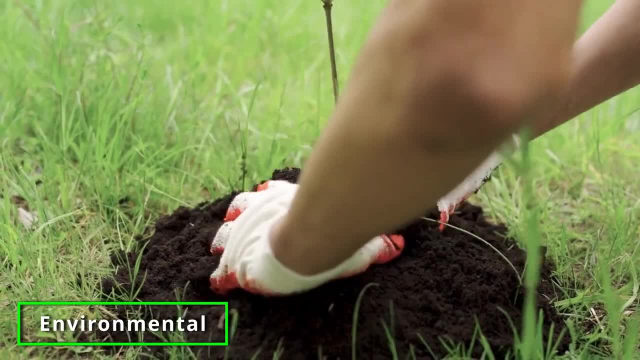 clear, necessary equipment is properly operated and maintained, and ensuring site safety. 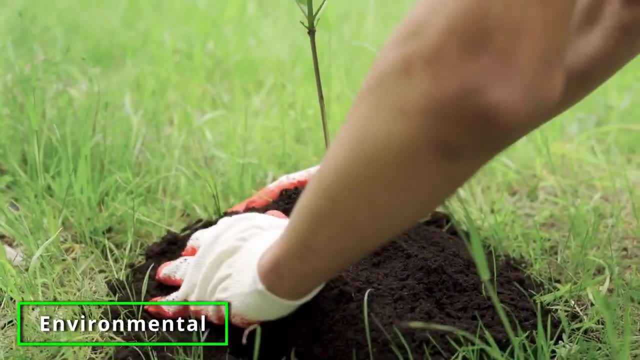 These jobs often cross over into natural resource management, and techs can be found working on many field-oriented projects in both branches. Entry-level environmental field techs had a 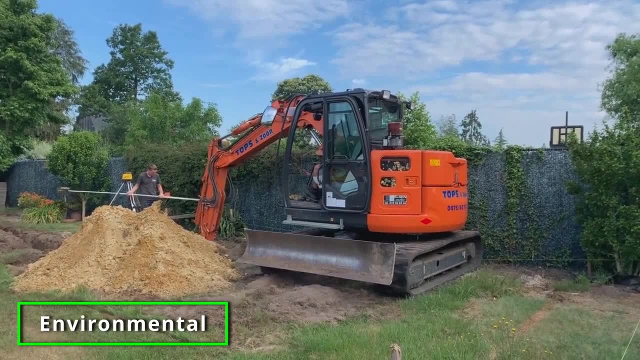 This job typically requires a bachelor's degree in earth science-related programs, but some employers will accept entry-level candidates with only a high school education 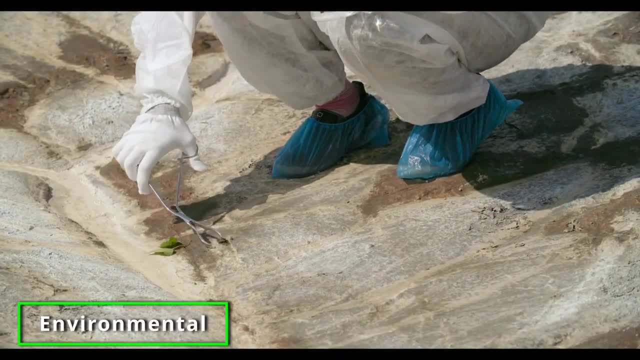 depending on their duties. On top of that, most of these positions require a HAZWOP or certification. Obtaining one of these prior to your search will make you a much more desirable candidate. 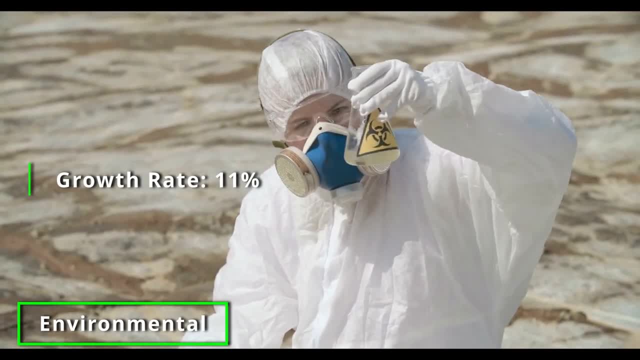 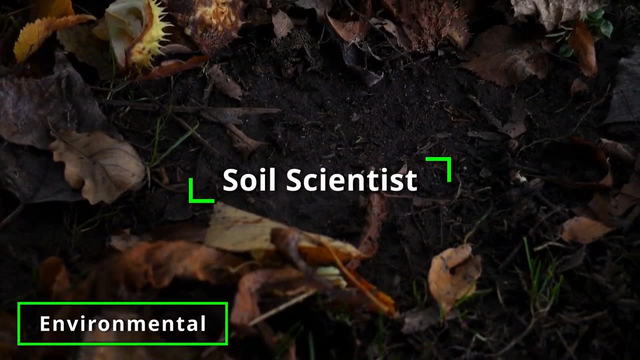 And lastly, this job is experiencing an above-average growth expectation of around 11% by the year 2030. Students who like to get outside and work with the earth will like to get out in the sun, and they will likely find soil science careers appealing. Soil science careers range 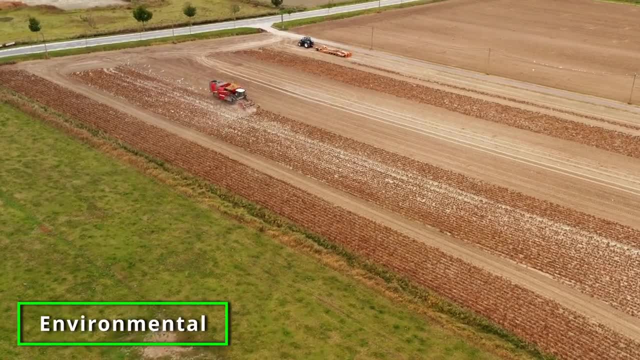 anywhere from looking at quality or efficiency of crop production to studying the formation of soils.